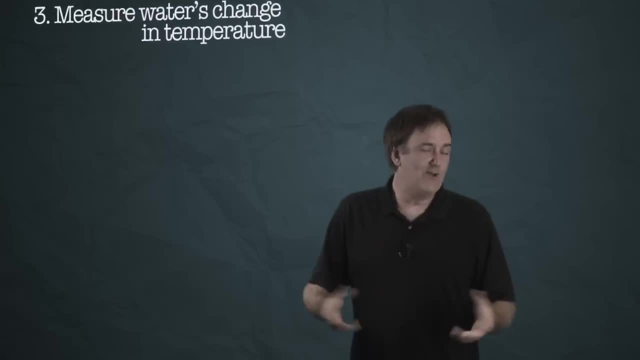 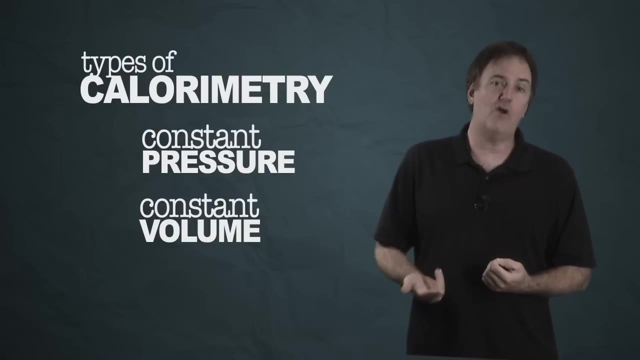 Now it does require a little bit of planning ahead. You have to build yourself a calorimeter. Now we have two types of calorimeters. We have constant pressure and constant volume calorimetry. I'll start with the easy one: Constant volume. oh, I'm sorry. constant pressure is the easy one. 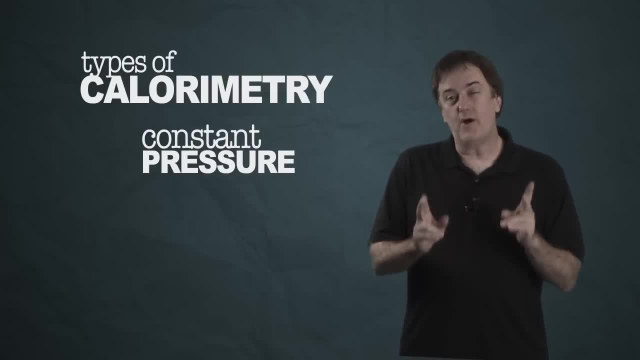 We'll get to the volume in a minute. Constant pressure calorimetry. we also call it coffee cup calorimetry, which will help you remember that it's super easy to make. When we say coffee cup, what we really mean is a cheap styrofoam cup. 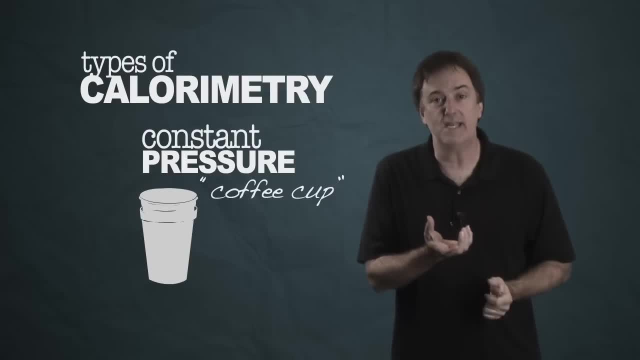 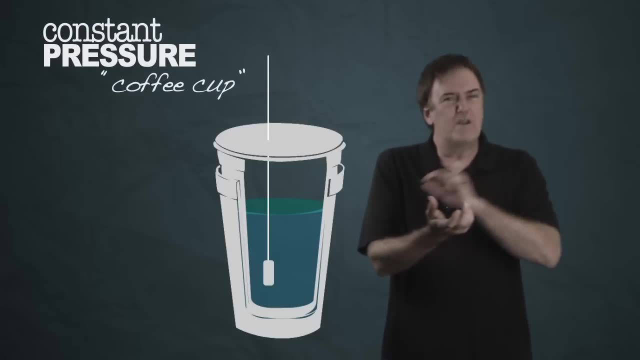 Heck go crazy. get two styrofoam cups and stick them in each other. You've got yourself the perfect coffee cup calorimeter. Fill it up with some water, Maybe put one of your reactants in. Maybe you put some acid in it, so it's got acid floating in your cup of water. 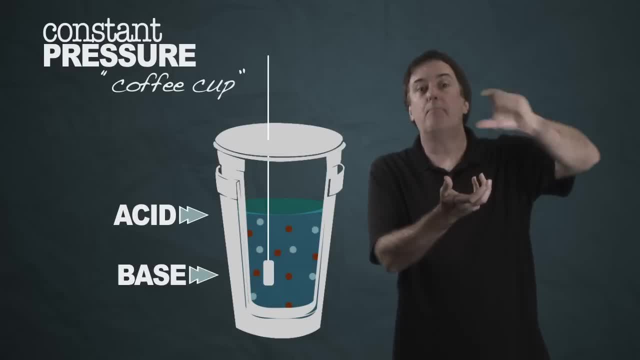 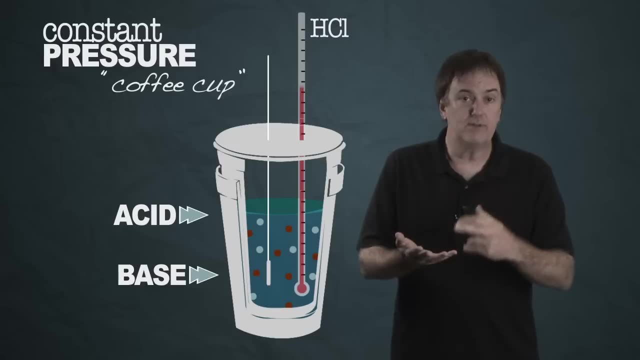 Now take some base, have a thermometer in it and pour it in Stir. That temperature will change, especially if you do something like hydrochloric acid plus sodium hydroxide. It's an exothermic reaction, so therefore it gives off heat. 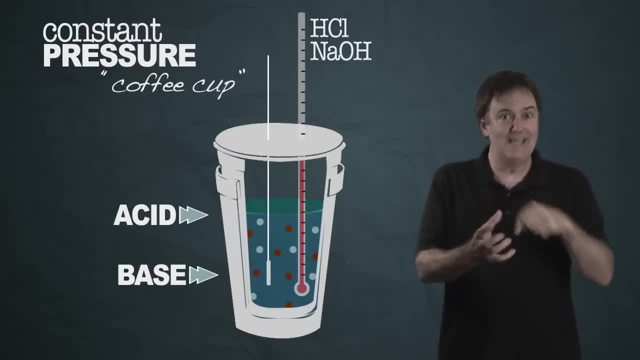 and sure enough, the temperature will rise in that solution. and it's real easy to measure the start and the finish. You look at the thermometer before pour it in stir. look at it when it stops. You've got yourself a delta T. 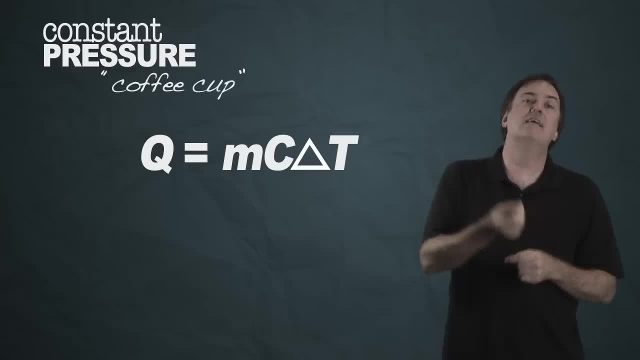 From that delta T. you simply multiply that by the heat capacity of the water, which is 4.184 joules per gram per degree C, and you multiply it by the mass of the water, which you can easily weigh by sticking it onto a scale. 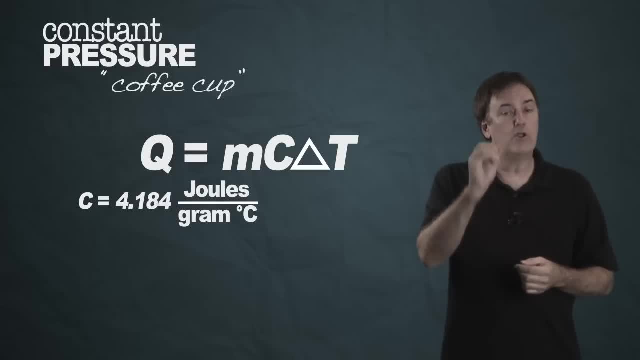 Put all that together and you've got your amount of heat, which we call Q. That amount of heat is what was released from the reaction. That's an extensive property. We know the amount. Now you divide it by how much stuff you used. 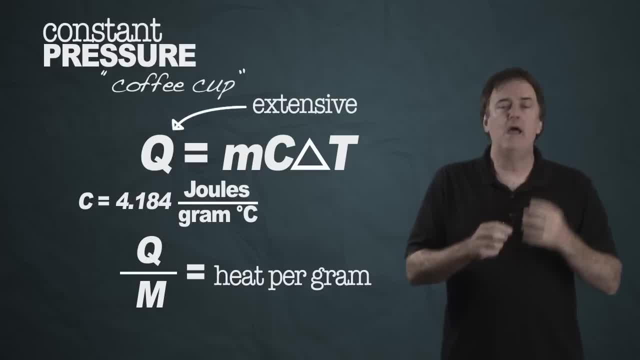 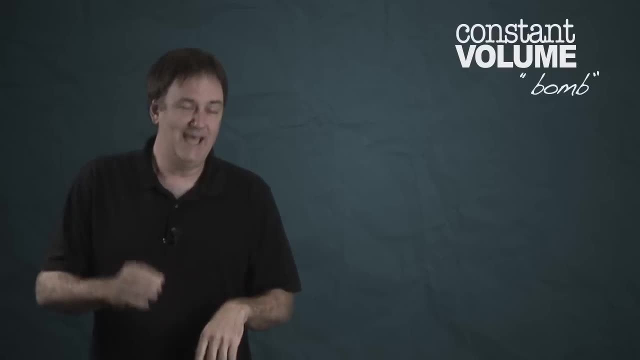 the amount of heat per gram or heat per mole, and you've got yourself the answer to the actual reaction you just ran. That's coffee cup calorimetry, Easy Cheap. Let's shift to constant volume calorimetry. We call it bomb calorimetry. 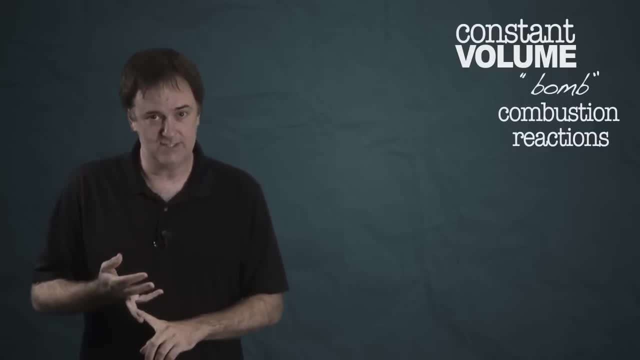 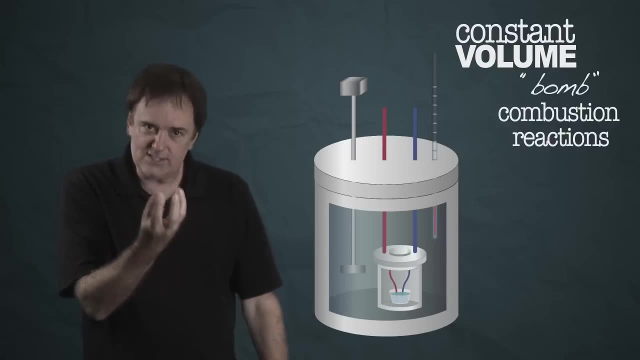 It's the classic way we measure combustion reactions. It's our favorite thing to put in a bomb. Why do we call it a bomb? Well, you take a stainless steel container. you put something highly flammable in it with a lot of oxygen. 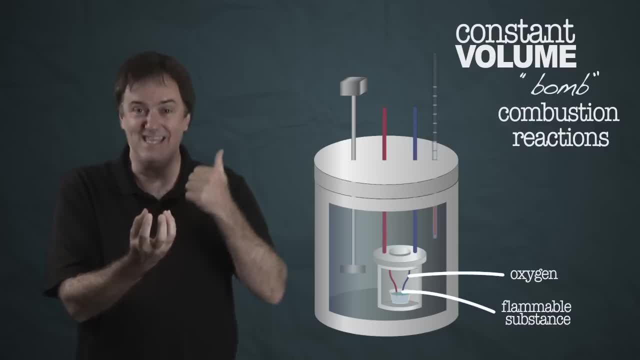 and you screw the lid on really, really tight and then you ignite it. Technically, that's what you do when you make a bomb. Now, for us, we don't want it to explode, so we make sure we don't use enough material to blow the thing to bits. 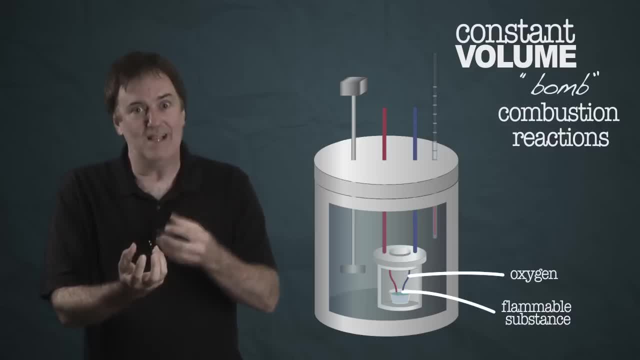 But we do use enough to make it get really hot inside. but the volume is set. so because the volume can't change, there's no work done, which means all the energy is dissipated as heat into the surrounding water. Only problem is it's going to cost you a little more this time. 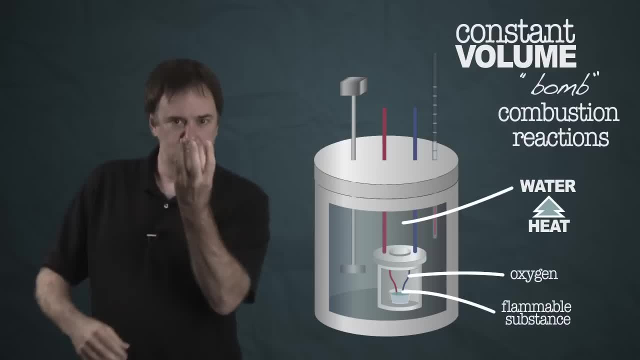 because now you need a big container of water, you need the stainless steel bomb, you need something to spark inside the bomb, basically a spark plug. you need wires on it coming out, you need a stir bar. you need all that apparatus hooked together. 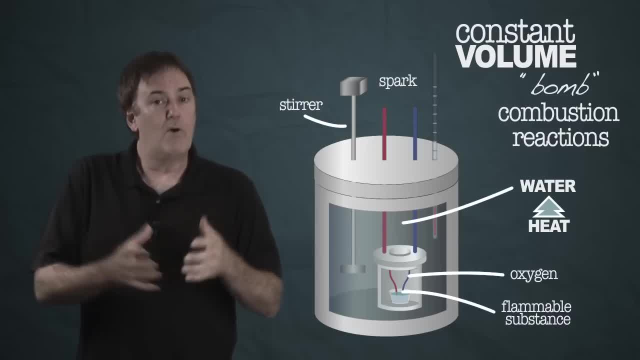 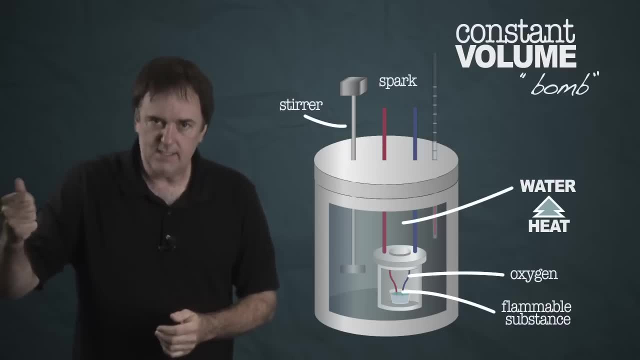 Oh yeah, an oxygen tank. you've got to put the oxygen into the bomb. But once you have all that and you've measured all your quantities, it's no different than the coffee cup. You push a button, it sparks, the reaction goes off. 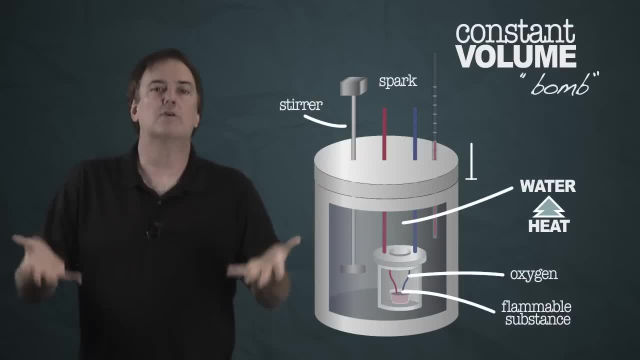 all the heat dumps into the water and the temperature climbs. Once again you've got a change in temperature that you can change into amount of heat. That's the basis of calorimetry. It works for bomb, it works for coffee cup. 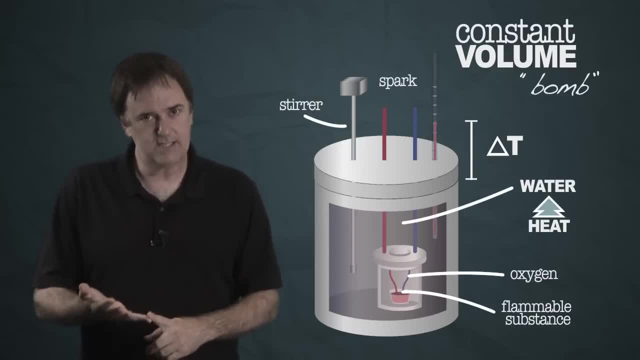 and that's how we get the values of delta H for a reaction and we get delta E for a reaction. So you'll see lots of problems in your book on calorimetry- and it's a really powerful technique- on how we get all these values in thermodynamics. Thank you.